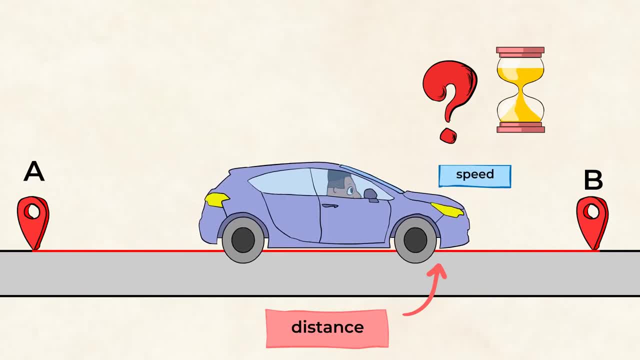 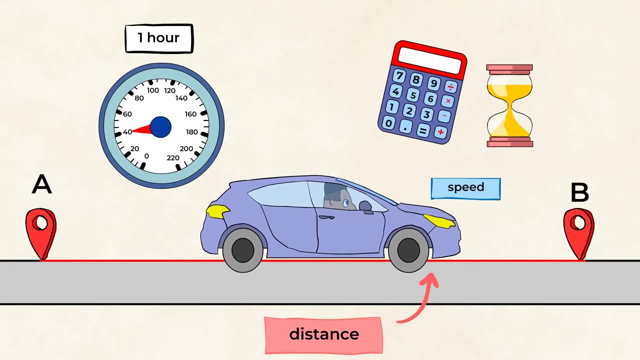 time. If you know the distance a car travels in a certain amount of time- let's say 40 miles in one hour- then you can also calculate the speed of the car. Sometimes the speed of a car doesn't change during its trip, So you can say the car is traveling at a constant speed, If that makes you. 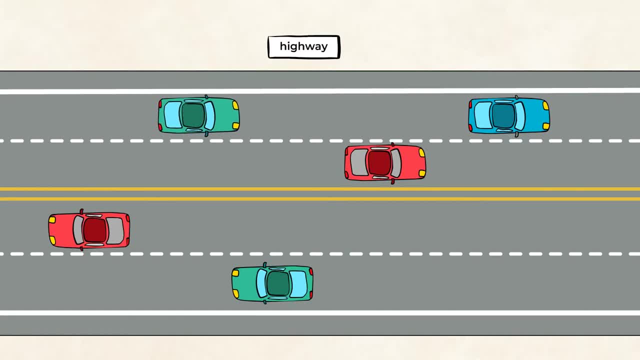 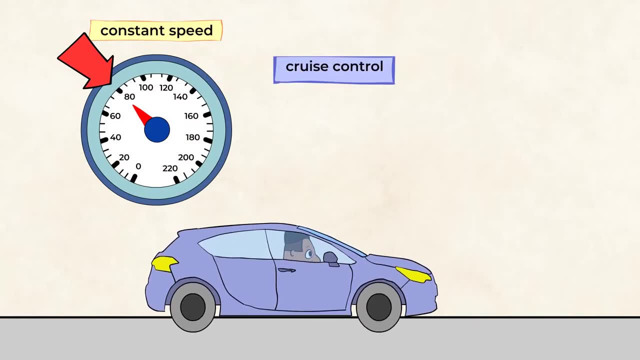 think about a highway. that's exactly the right idea. That's a place where a car can travel at a constant speed. You've probably heard of cruise control. right, It's a setting you can use while driving a car And the car then drives at the same speed. 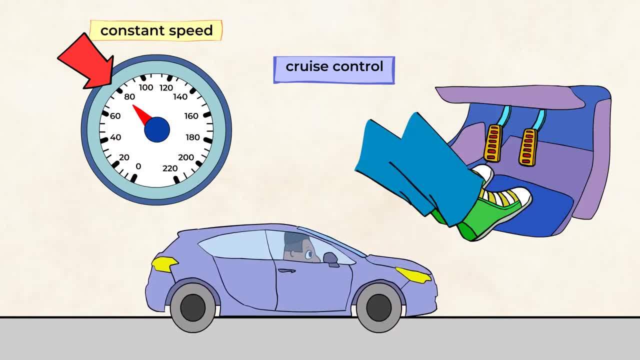 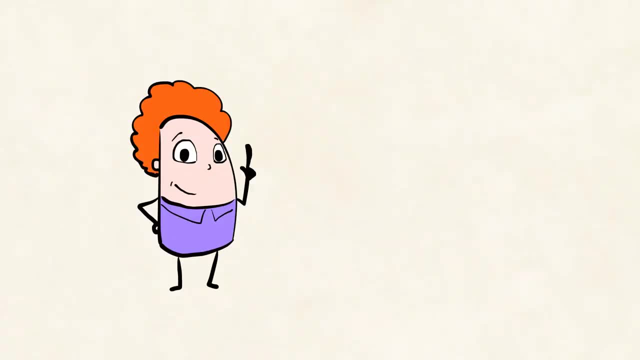 even if your foot isn't pressing on the gas pedal. If you're using cruise control while driving, your car is traveling at a constant speed. Most objects don't move at a constant speed for very long, though You don't move at the same speed either. Just imagine how many times you slow down. 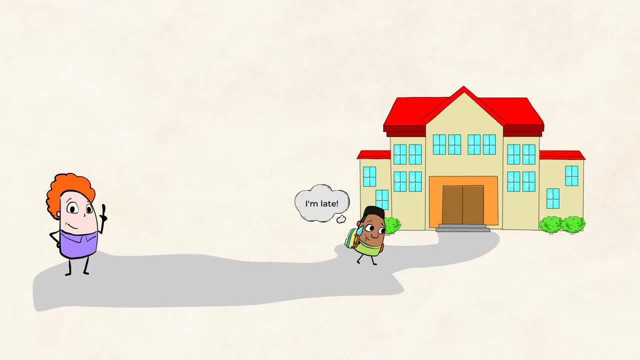 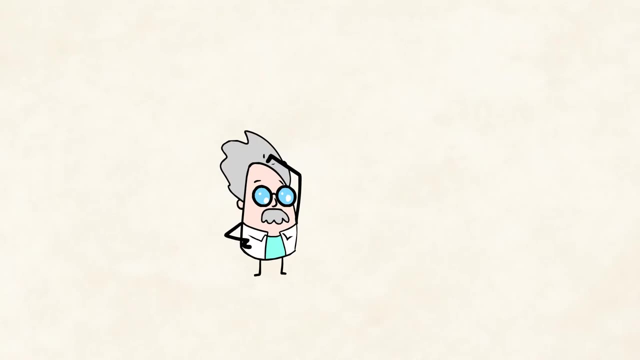 and speed up on the way to school, Especially if you're running late for your first period and dodging all the other people in the halls. Moving objects change speed many times while in motion. Think about your father driving the car on a highway using cruise control. If there's an accident or a traffic jam up ahead, he may have to. 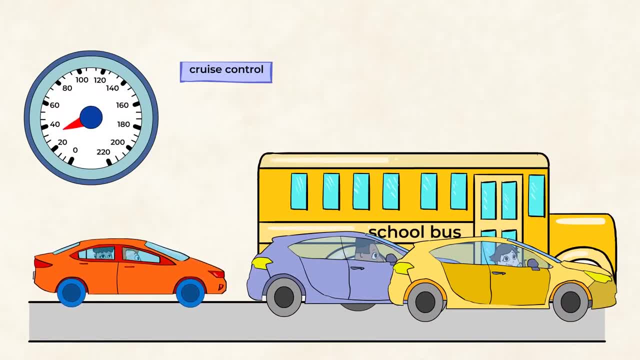 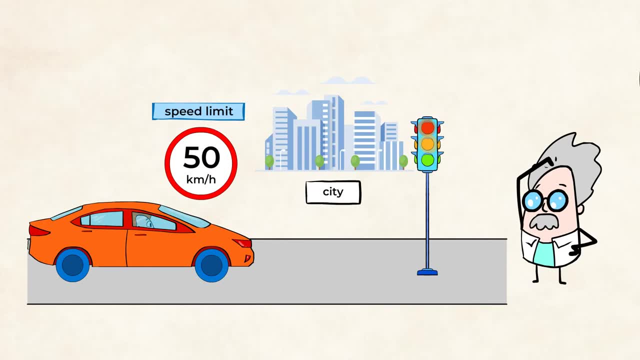 change the speed and slow down or even stop the car. The speed of your car in the city may also depend on the speed limits or depend on traffic lights. You may need to stop at a traffic light if it's red, Or you might want to speed up to pass another car. There are other examples. 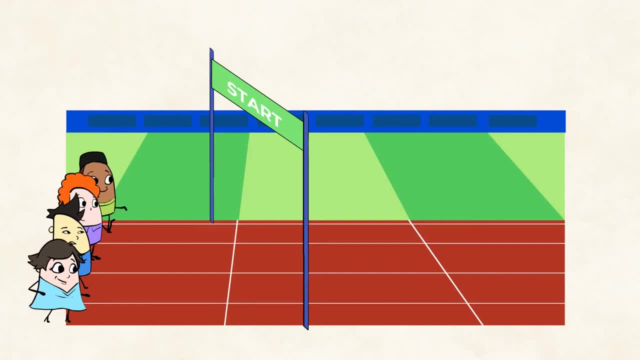 Marathon runners don't run at constant speeds during the entire race. At the starting line there are many runners all crowded together and they have to move more slowly. But as the crowd thins out, a runner can increase their speed. A runner may also slow down. 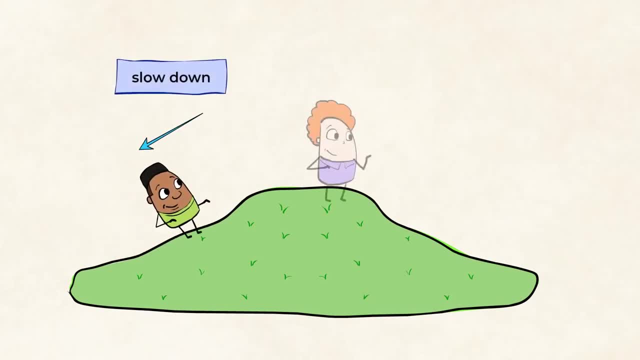 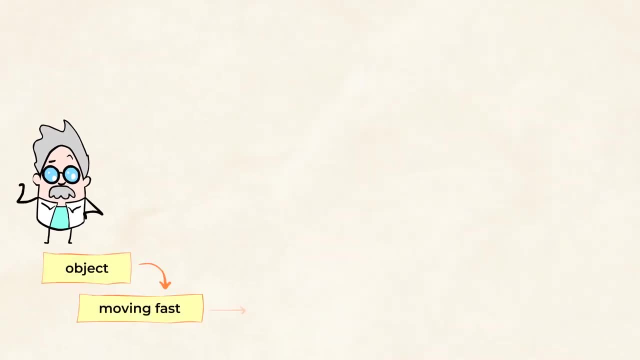 when going up a hill, or they may increase their speed when going down the hill. It might seem obvious, but if an object is moving fast, it can travel distances in a short amount of time. Just imagine the fastest runner in your class and the slowest one. Both of them have to run the same distance.